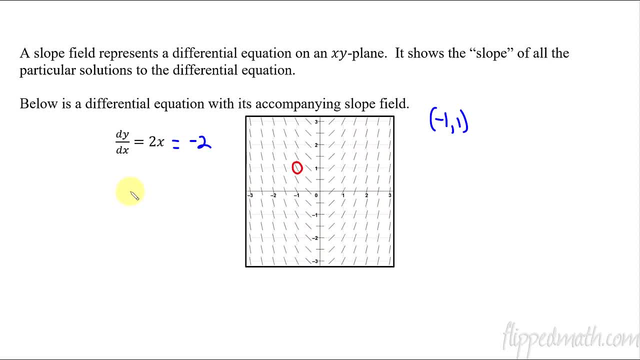 figure that out for every single little piece of these. And if I took the antiderivative, just so you know, this would give me. the antiderivative would be y equals so x squared 2x squared over 2,. 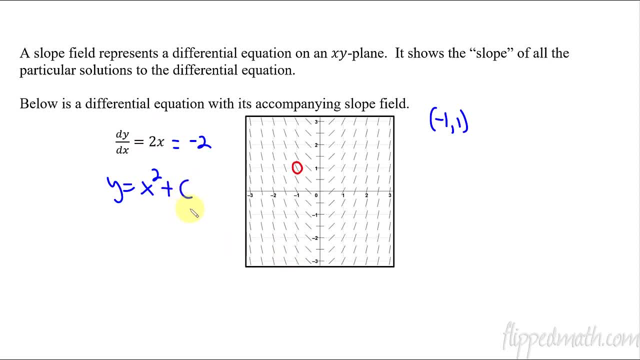 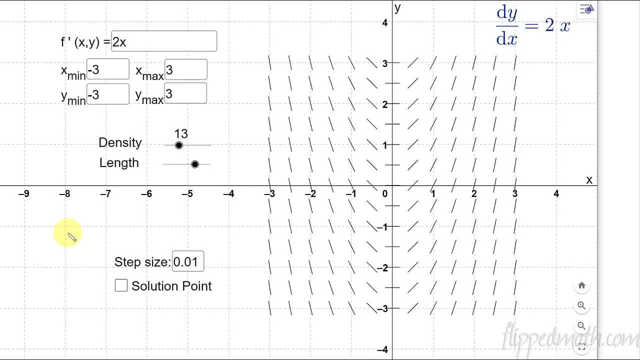 so the 2s cancel and then plus c. So the plus c is the general solution. You remember that We have our general solution, So this slope field represents any possible c. Now let me show you this on a cool little app. This thing was used using GeoGebra, GeoGebra, And it's on a. 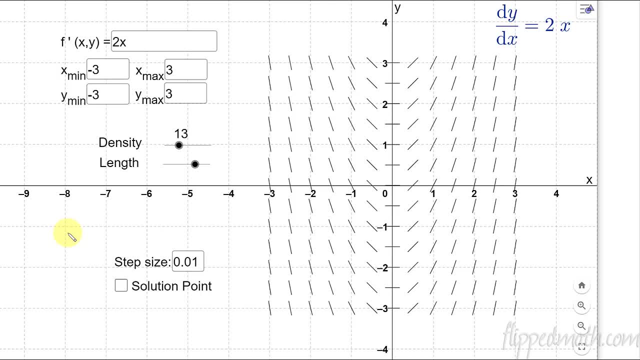 website. So if you're on FlipMath calculusflipmathcom underneath our video, if you scroll down, you'll see this thing there And you can plug in any little differential equation you want here and it'll show you the slope fields- Pretty cool stuff. So what this is is I could now take my differential. 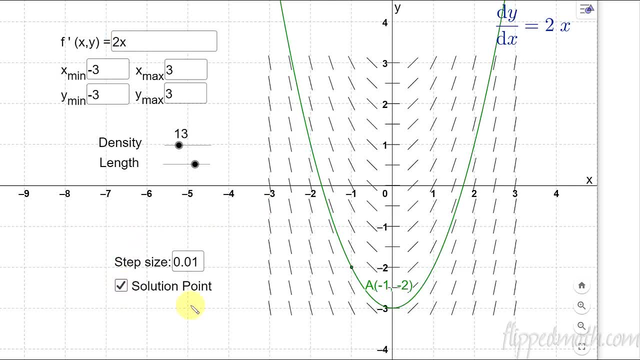 equation of 2x, and I'm going to click this thing here- plot a solution point. This is where you have all the different plus c's. There's an infinite number of them, So I could just go up and down and, you see, this creates a parabola which would make sense. 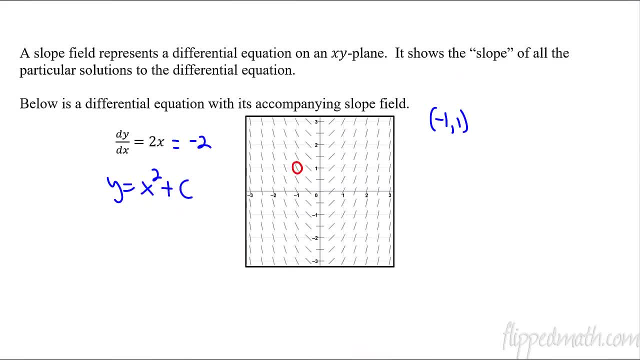 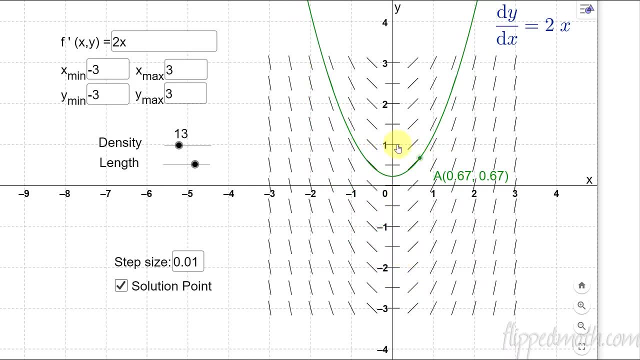 Because we said y equals x squared plus c, was our answer. So it's just x squared plus c. So any plus c we want. That's what's going on with this thing, And then you can see these little solid hash marks. That's where we have the minimums and all this cool stuff. So that's what we're doing today. 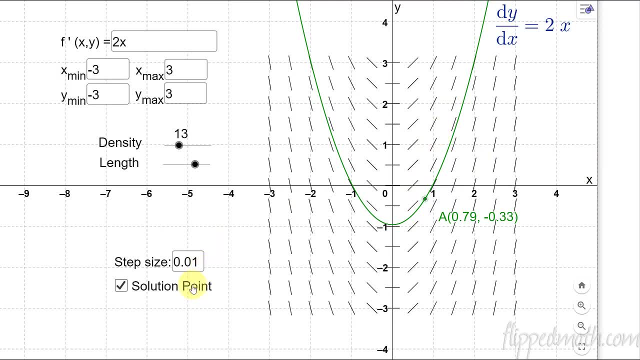 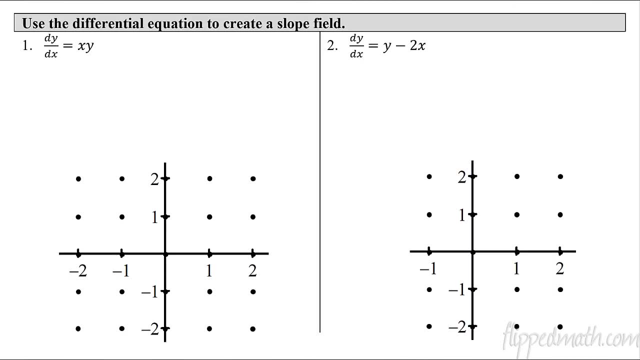 is figuring out how to graph these little hash marks. You don't have to worry about the exact solutions, what I have in green. We will do that in our next lesson, So let's graph one. So this is how we start. Sometimes you can just look at this: If it's x times 1, you can just look at this. 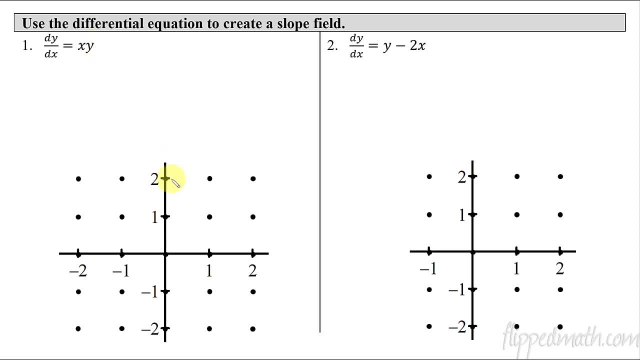 Why You think okay. well, if I just choose any random point like 1, 1, this point right here, 1 times 1 has a slope of 1.. So I'm going to have, as I start to draw, this, I actually want to focus. 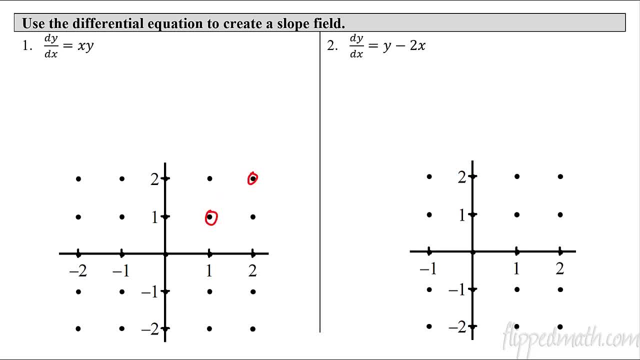 in on the slope. I'm going to look at this point and this point as I'm drawing it. So then I know it has a slope of 1, and I'm just kind of putting a hash mark right there that would eventually connect them if I wanted. Okay, so I don't actually circle them, I'm just thinking about. 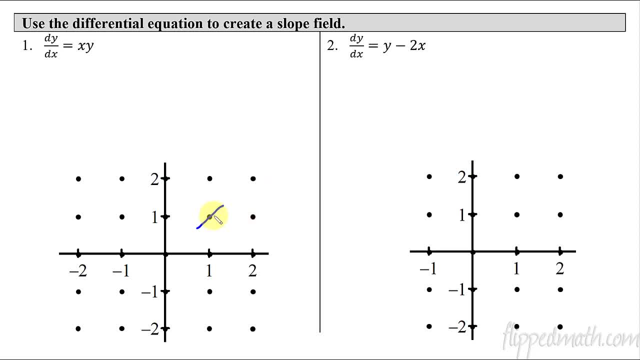 that, as I'm drawing it myself. So then I get the hash mark with a slope of 1.. And then you just do this for every single point. Well, what about the easy ones? How would you get a slope of 0?? I like. 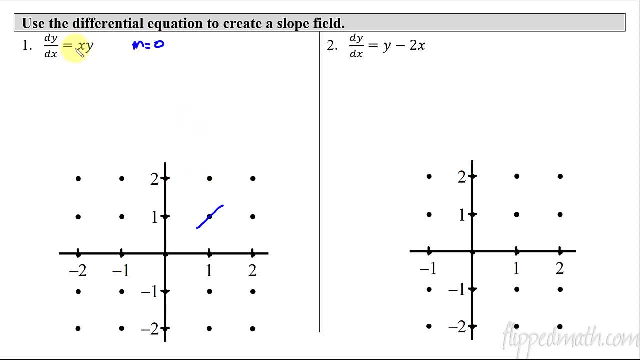 to do that because they're easier. A slope of 0 would be if x was a 0, right, So I can go ahead and say: if any of the x's are 0, so all the points with x 0, we have a flat hash mark there. And if 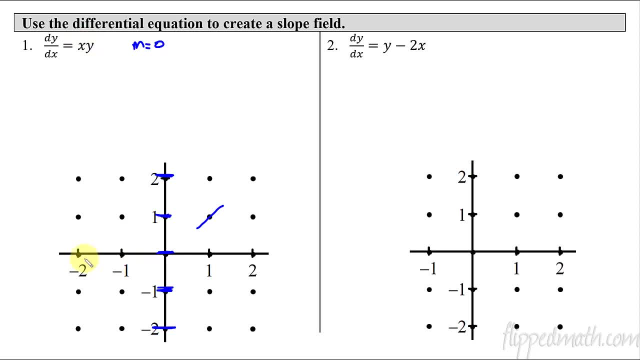 any of the y's were a 0,, right, Because something times 0 will give you 0 here. So all of these along here with a y value of 0,- and I know it's probably hard to see on your graph because it's- 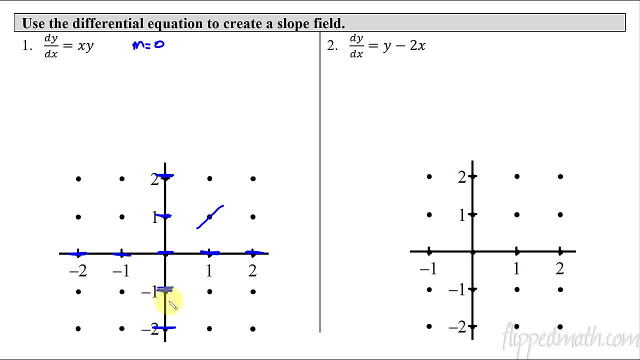 right on the axis. So I'm going to go ahead and do that, And then I'm going to go ahead and do this. It's hard to tell, But those are all the slopes of 0.. So now, from here we just start. 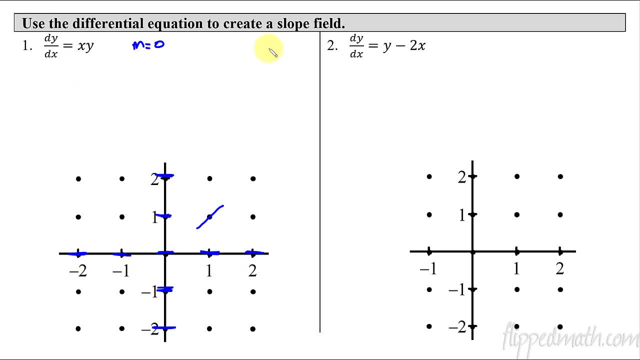 filling out the rest of this. I'm going to show you that there's a chart you could make. I'll do that on this one, the second version, But sometimes it's just quick and easy Ones like this. it's quick and easy to just do it So like negative 2 comma 2, that's just negative 2 times 2.. So 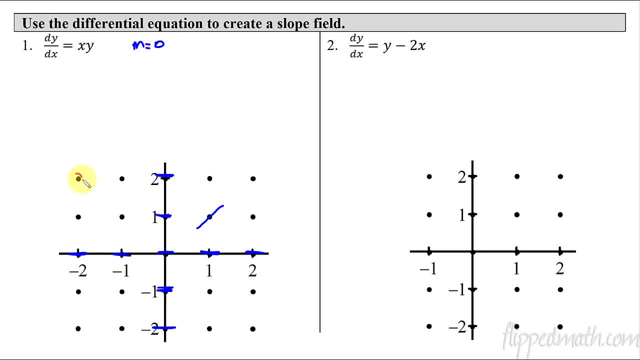 negative: 4.. So now, what I do there is: I'm eyeing it, I'm starting at this point and I'm going 1,, 2,, 3, 4 down to here. These do not have to be perfect. Okay, you're just eyeballing it, So I'm. 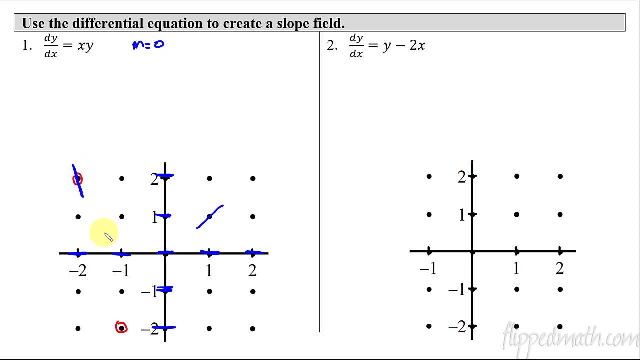 going down to there. So I'm making a line. Looks like it would have a hash mark of a slope of negative 4.. This one here, negative 1 times 2, has a slope of negative 2.. 1, 2 would have a slope of positive 2.. 2, 2 has a slope of 4.. Again, 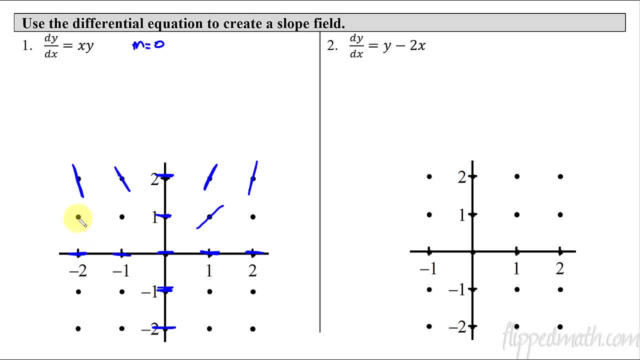 I'm just eyeballing it. So it's a pretty steep slope. Negative 2, 1, slope of negative 2.. So you draw your hash mark with a slope of negative 2.. Negative 1, positive 1 has a slope of negative. 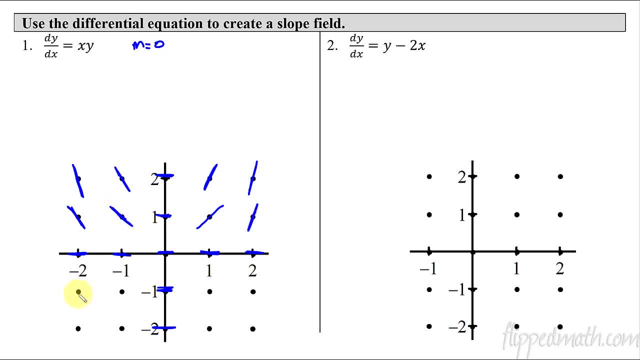 1.. Keep going here. 2, 1, slope of 2.. And now we're down to the negatives. Negative 2, negative 1 is a positive 2.. Negative 1, negative, 1 is a positive 1.. 1, negative, 1, negative 1.. 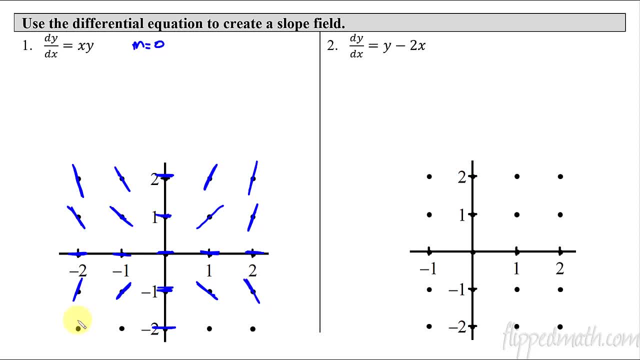 2 times negative, 1, negative, 2. Negative, 2 times negative, 2, positive 4. What's that? one Negative, 1 times negative, 2, positive, 2.. 1 times negative, 2, negative, 2. And then 2 times negative. 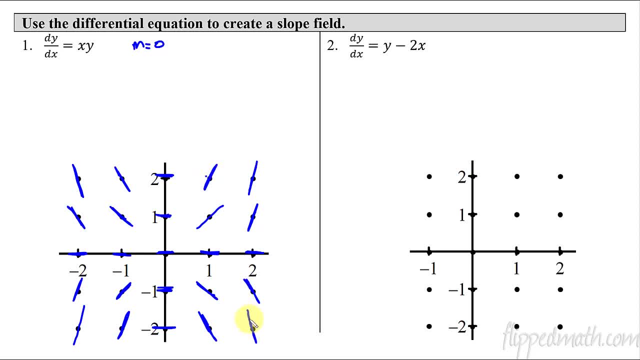 2 is negative 4.. So again eyeballing it way up to that dot up there: negative 4.. Okay, so this creates our slope field. Now what does this do again? This gives us the slope of the original solution of what y equals. It's the original graph before you took the derivative. 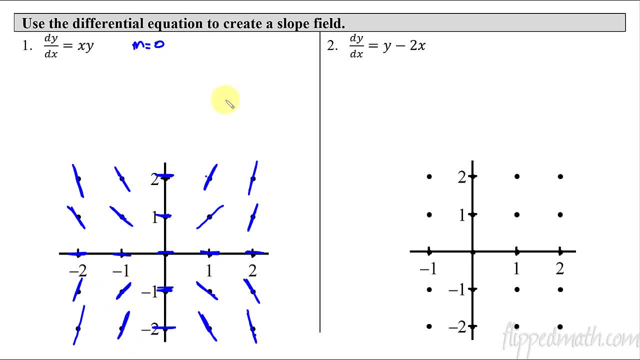 This gives you the slope And the nice thing is it gives you a little bit of a picture of what's going on. Your graph here. you can hardly tell anything Like: what the heck? What is this graph? You can't really see because we don't have very many points and you don't have very many hash. 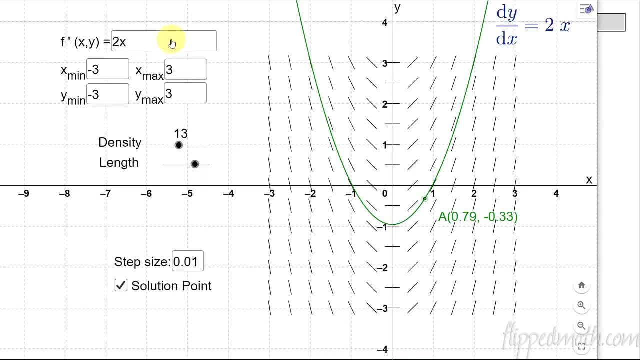 marks. So let me show you on our little GeoGebra tool. I type in xy and hit enter So you can see here this is larger and it has more hash marks, these little dashes. So you get a lot better feel for what the graph is doing. And I can even manipulate this. Instead of 13 density, I can. 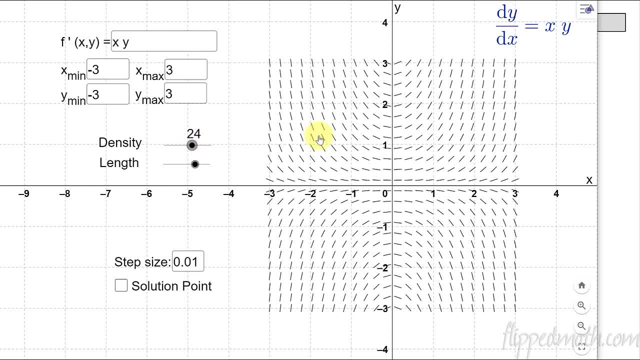 bring it up and I get more and more hash marks. Oh, that's cool, Look at that Cool. So you can get a lot better feel for what's going on with the more hash marks you have on a slope field. And then I'm going to plot my solution. 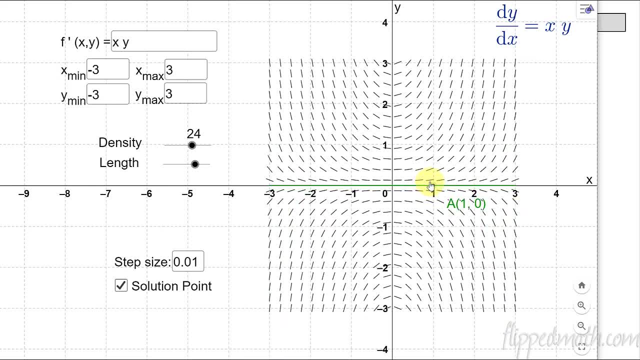 point, And you can see here these are all the different types of graphs that it could be. So this again, slope field, is all of the graphs, So it's a general solution, not just one particular solution. Okay, I also like to think of this. let me get rid of that. I like to think of these as 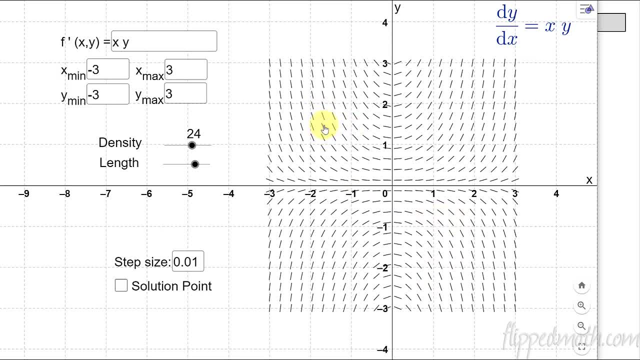 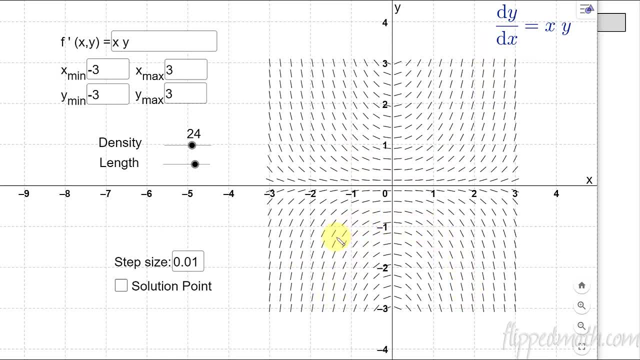 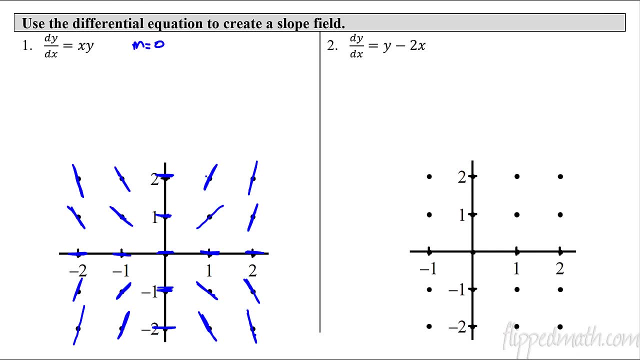 to think of it as the current that pushes it one direction And then so these lines just kind of push it, flattens out, flattens out, pushes it back down the other way. All right, let's do another one. This one you're going to do on your own, but before you get started, let me help you. Sometimes 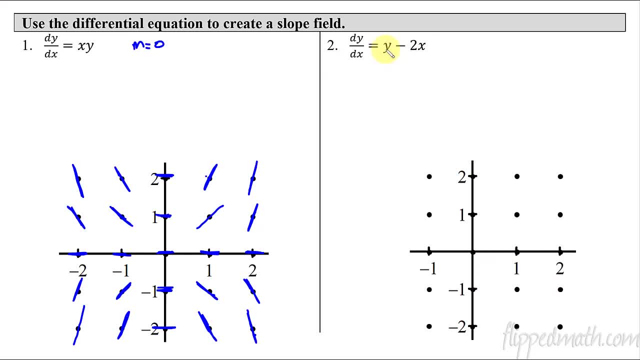 it's not as easy to just think of one comma, one plug in the values and do it. There's a lot to keep track of, So a lot of people like to make it a little bit more complex, So I'm going to do a little. 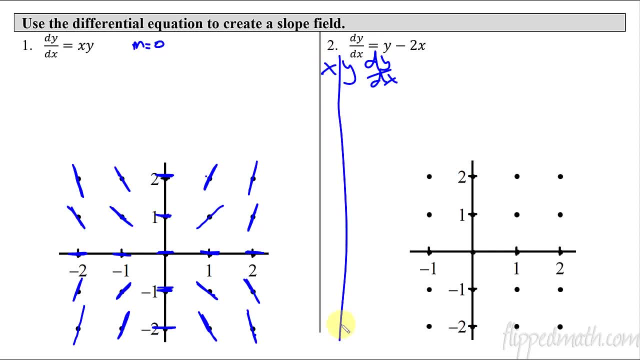 bit more complex. So I'm going to make a chart like this. So I'm going to go x, y and then dy, dx, And so what I do from here is: how about I just take this whole column? here all the x values are: 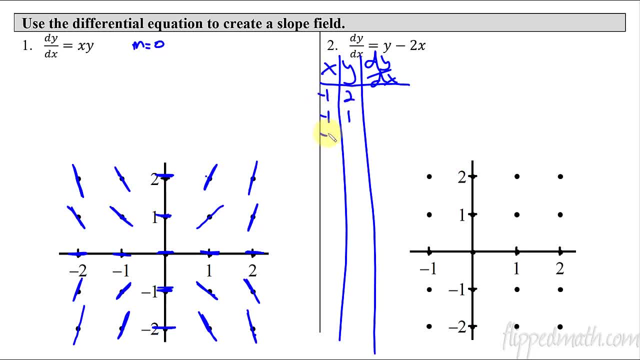 negative one. so negative one, two. negative one, one negative one. zero negative one. negative one, negative one, negative two. Okay, so now what we can plug in this x and y into this thing which is here. So it's going to be a two plus two slope of four. one plus two slope of three. Okay, 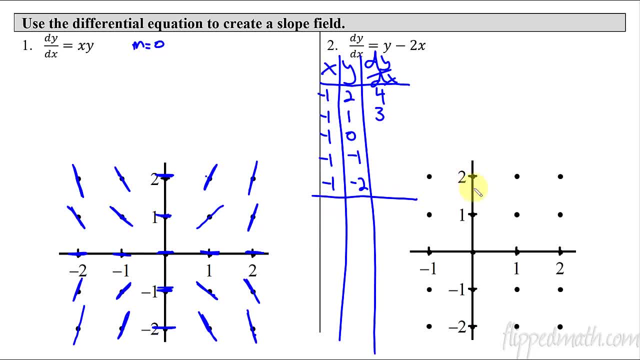 so this is how it works, And then you just keep going here, And then I would even now start my new column. So x is of zero, zero two, zero one. So keep filling this out, And then, in fact, 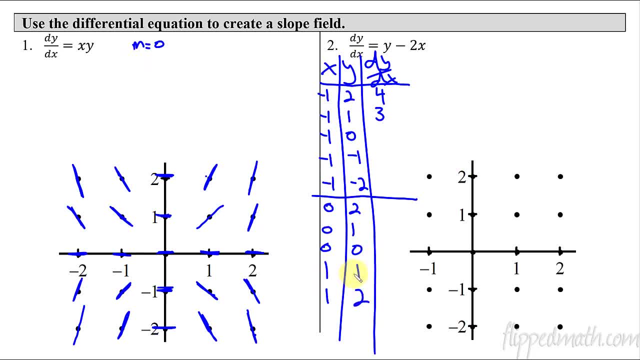 I want you to go ahead and pause the video now. Pause this. Oh, negative one, negative two. So pause the video. try this one on your own and let's see how well your hash marks match up to mine. Here I have my answers for my slope fields. I noticed that I had put the wrong numbers here. 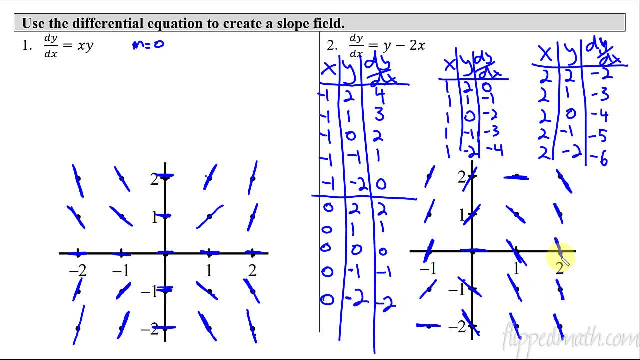 Some of you probably caught that, So I got this fixed. And here's the thing: when you graph these like let's be real negative six, negative five, negative four, trying to graph a little hash mark of that slope, That's crazy. You're not going to be able to be exact, accurate on that, Okay. 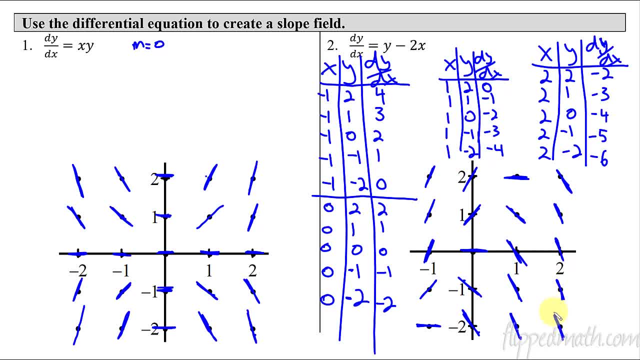 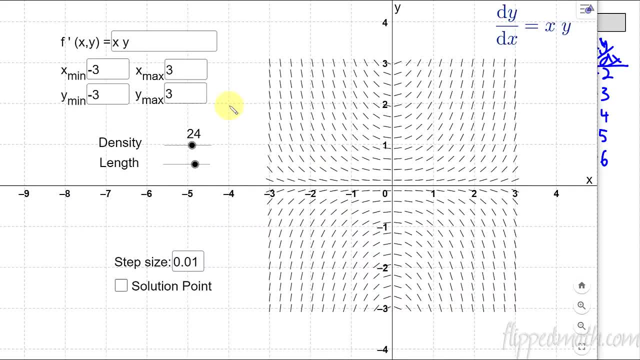 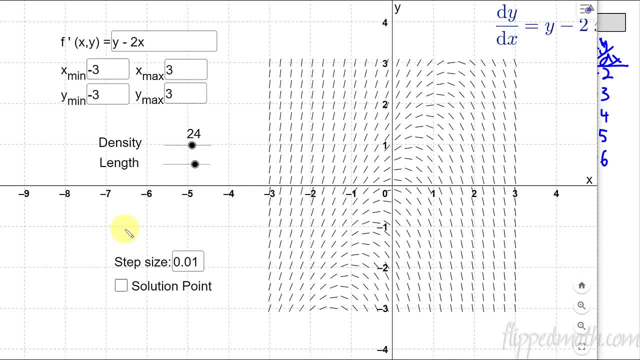 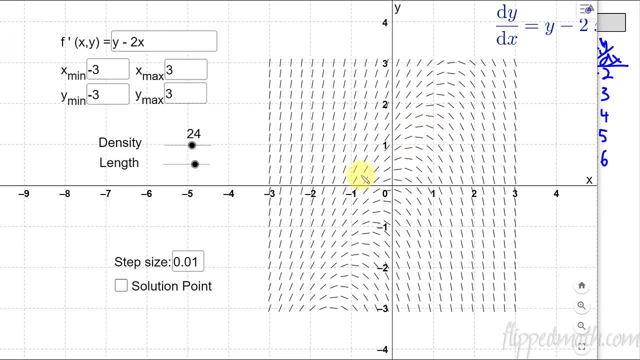 looks like If you were to just plot a point somewhere, you'd see the current, take it up, up, up, up and then turn around and come back down. So let me show you what this looks like. So this is the graph, So it could be going up here. These are all the possible different. 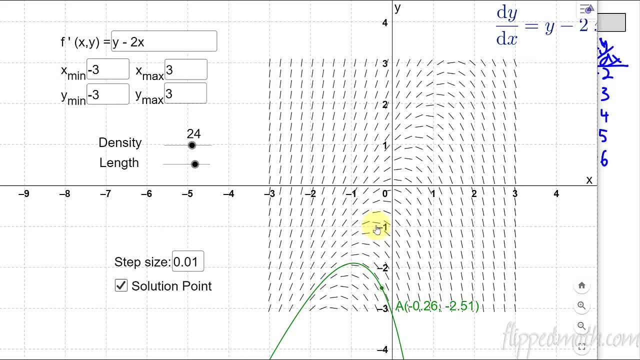 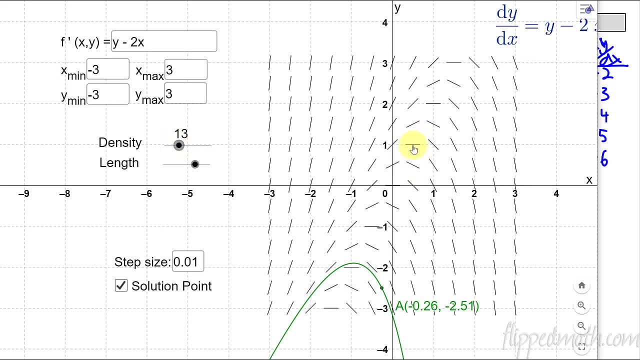 graphs that you'd have. But notice every place where you have a horizontal line. I have too many hash marks here. let's go back to I like 13. 13 gives me a hash mark right on the little half marks and on the coordinate points, so you can see I'm going to make it match up right there, boom. 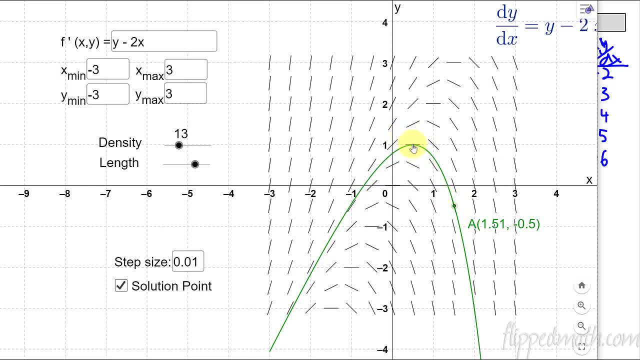 see that you've got the maximum right there where there's a horizontal hash mark for your slope field, and that's so. all of those represent maximums all across there. okay, again, this lesson, you don't have to sketch any type of solution graphs. we'll do that in our next lesson, next up. 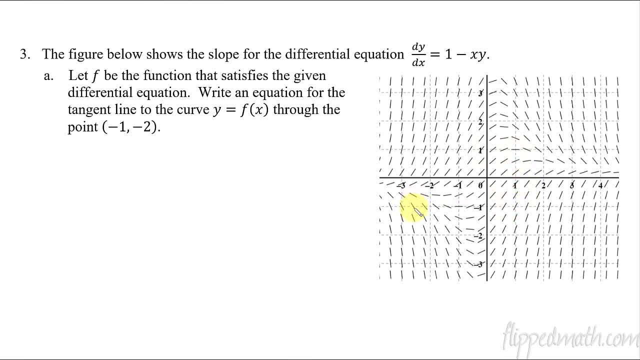 we have this differential equation with its accompanying slope field. this one's kind of cool. I like this one. you can see here, if you just picked a point anywhere on here, you can see that it's going up, coming back down, like it's kind of coming down here like this and then so it would. 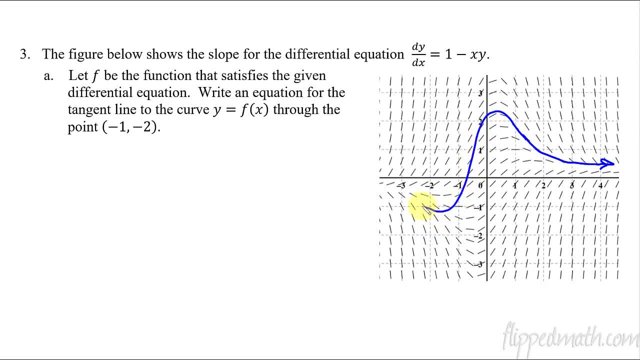 come up, but then it would turn around and then maybe come back down and then back in this direction. okay, so it's doing some weird thing like that. so all we're doing now is we're just going to write an equation of a tangent line at this point: negative one, negative two. let me circle it so. 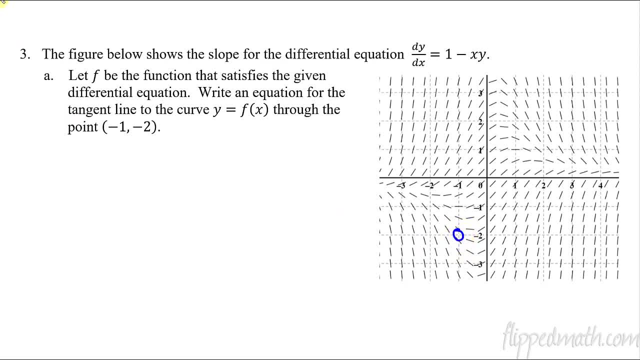 I don't have a hash mark there, but right there. negative one, negative two. let's figure out what it is. so here's the derivative one minus x, y. that differential equation will let me figure out my slope, so I plug in a negative one and a negative. 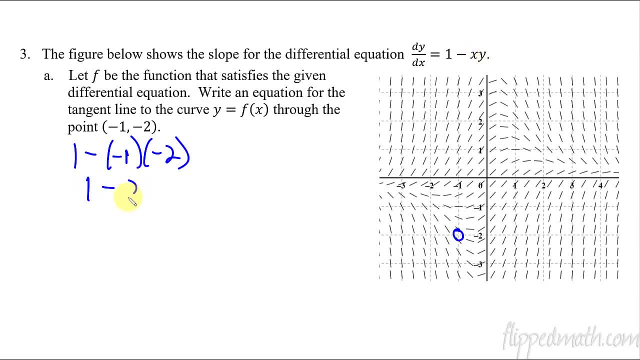 two into the x and the y. so that gives me one minus two or negative one. that's my slope. so then I just use the coordinate point y. oh wait, let's do this first. so the slope is a negative one. right there, get rid of my circle. so my equation of my line is: y plus two equals. 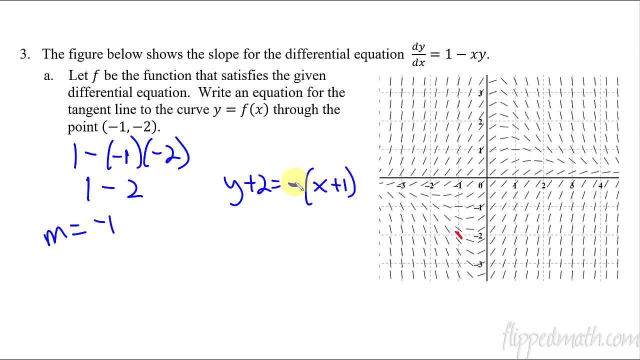 slope of negative one times x plus one, using point slope form with negative one, negative two. so there's my equation of the tangent line, and then that means that line would have a slope of negative one. so it'd be looking something like this: and now can you visualize what that would look? 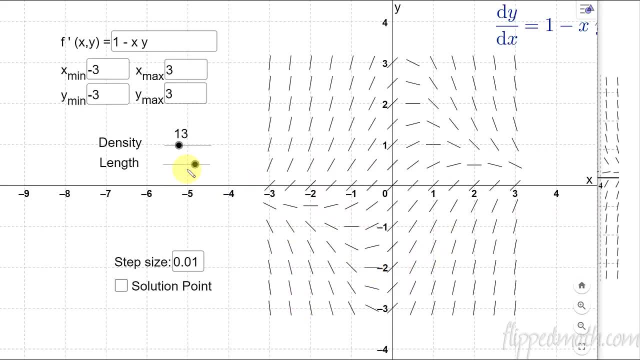 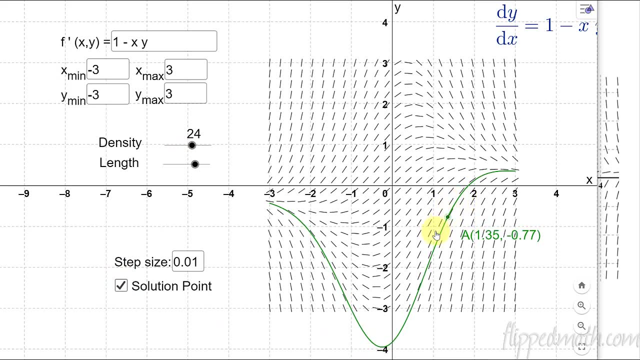 like let's go back to our GeoGebra app. so here's the same graph. I'm going to put a little bit more dense so you can see more of it, and then our solution points. so you can see here if I drag it to negative one when it腑. 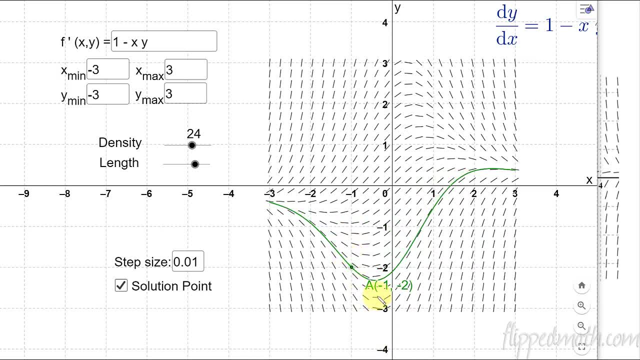 negative one, negative two, right there, boom and then. so now you could visualize the tangent line that we drew on ours. that's how that would match up right there. that'd be a tangent line. okay, pretty straightforward. you actually don't even need the slope field for this, but we're doing. 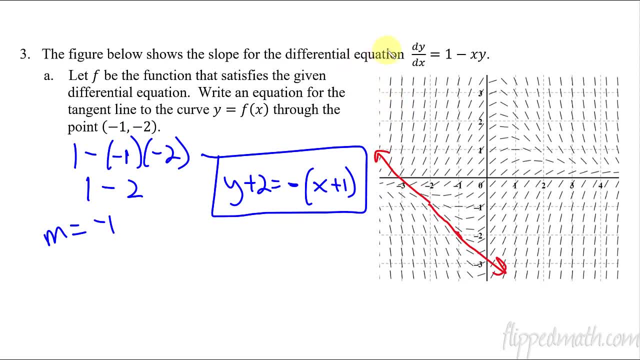 i'm showing you how to do this because often on an ap exam, when they introduce differential equations to a problem, they'll have something like this where you do a tangent line and then there's a slope field going on. that you'll have, but we'll do more of that in our next lesson, okay, 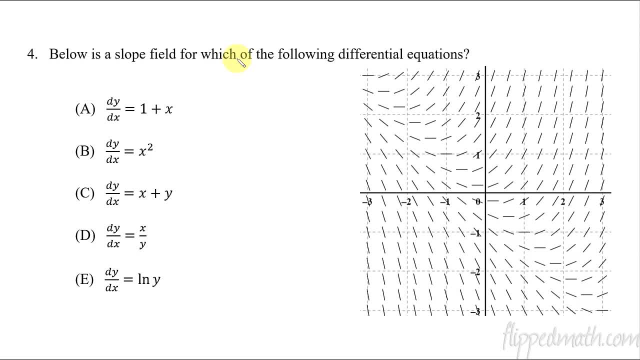 last one. now we are starting with a slope field and we're going to try and work backwards the other way. so here's our slope field and which one of these matches up. so there's a few strategies for doing this. i like looking for horizontal hash marks and vertical hash marks. this thing doesn't. 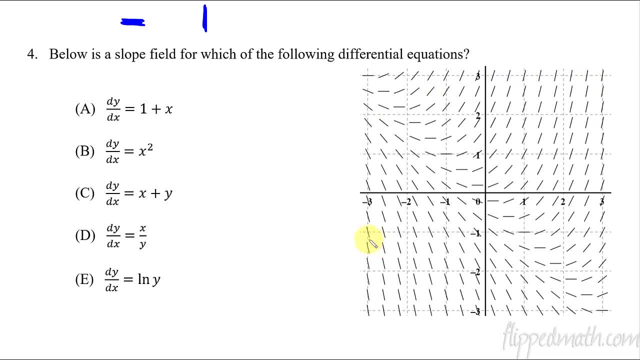 have any vertical hash marks. it gets close, but there are no vertical hash marks. so what that tells me? that's an important thing, because if i don't see vertical hash marks, see this one right here: if y was zero, you, this derivative does not exist, and i would have something going on at y equals zero. so all across. 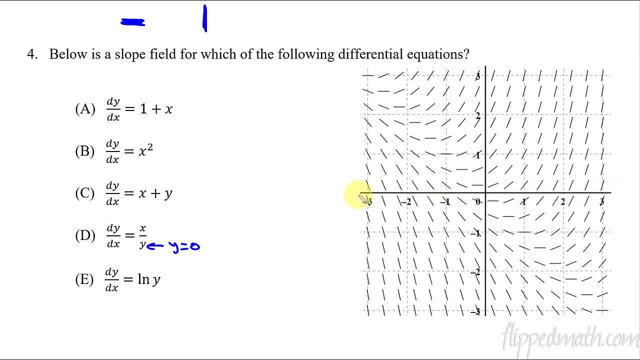 here. i would have a vertical hash mark most likely, or else there would be no hash mark at all. usually it's a vertical hash mark, is what that is. i know it's not going to be this one, but i'll show you why. else here in just a second. also notice, do we have any? uh, horizontal, yes, we do, i've got. 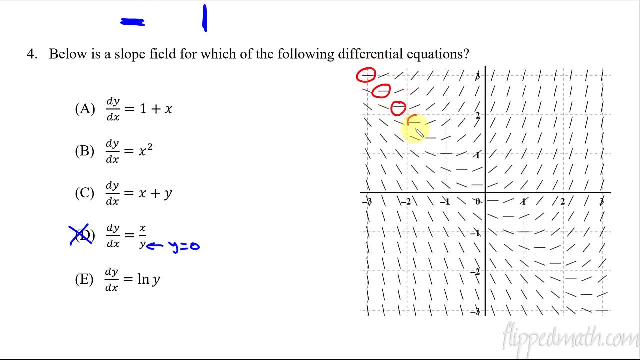 a horizontal there and there and there and there. so it goes on this diagonal line: y equals negative x. right y equals negative x, this horizontal line all the way down here. so what's important is that means that if x and y are opposites. so i'm going to make a list of 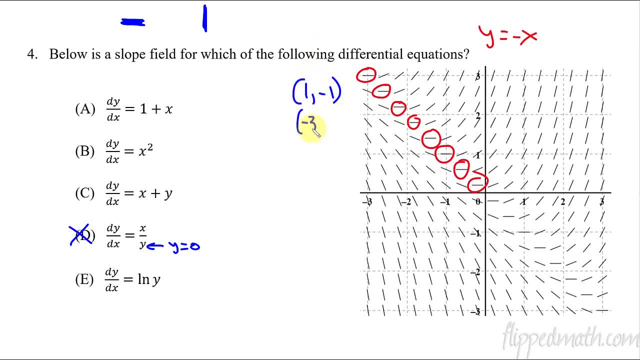 numbers that are opposite: one and negative, one, negative three and three, or i could say three and negative three, like those are all just opposites. if they're opposites, then that means you will have a zero slope, a horizontal tangent. so take that knowledge and let's plug in some points. 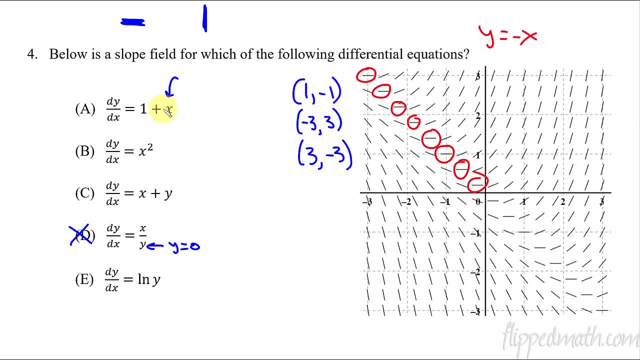 if we plug in an x value of one in here and then y is negative one, this doesn't equal zero. okay, so it's not that one boom. plug in a one here. one squared is one we want. if we plug in a one negative one, it should be zero, not that one. that was easy. this one, plug in a one plus a negative one. well, 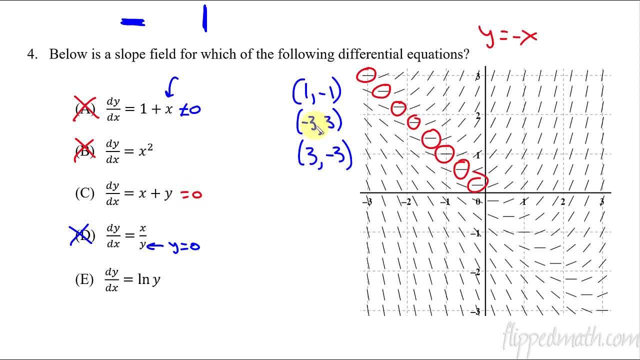 that equals zero. that would equal zero. try these others: negative three, three negative three plus three is zero. oh okay, i'm gonna put a little happy face next to this one, because i think that's probably the right answer. we've already showed you why here. but if you again, if you plug in a one and a negative one,